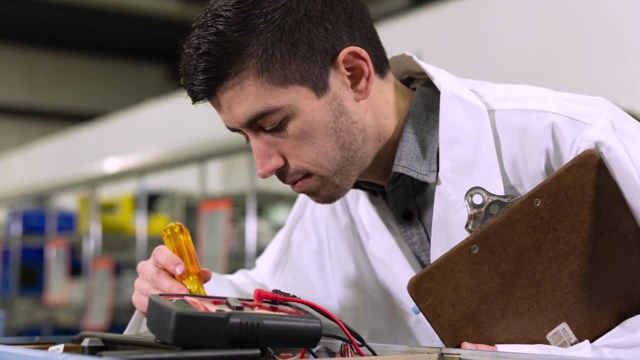 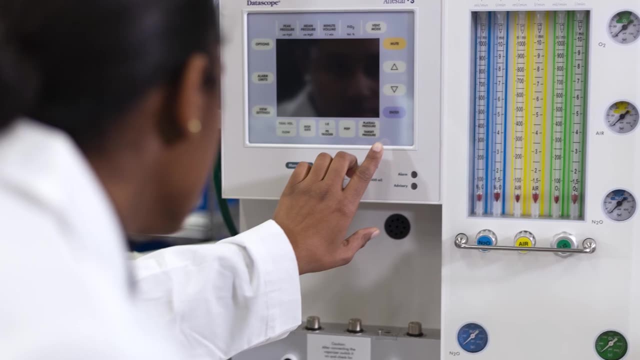 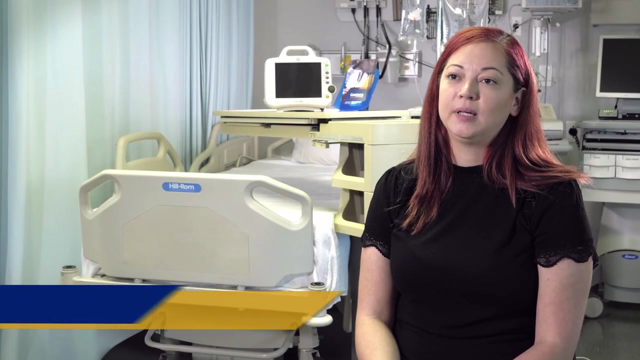 I feel like biomedical technicians or engineers kind of get lost in the health field. People kind of forget that somebody needs to make the equipment work and make sure it works properly. Hi, I'm Regina Cruz. I am the Biomedical Equipment Technology Program Coordinator for Centura College. 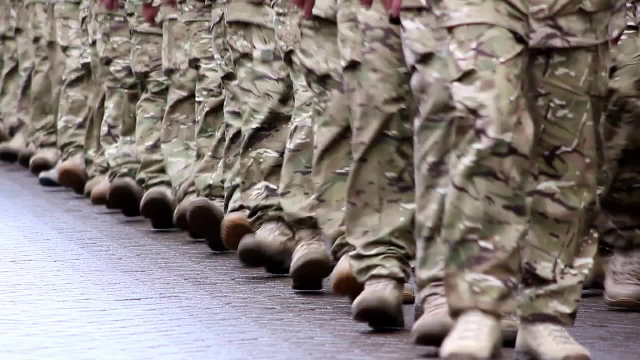 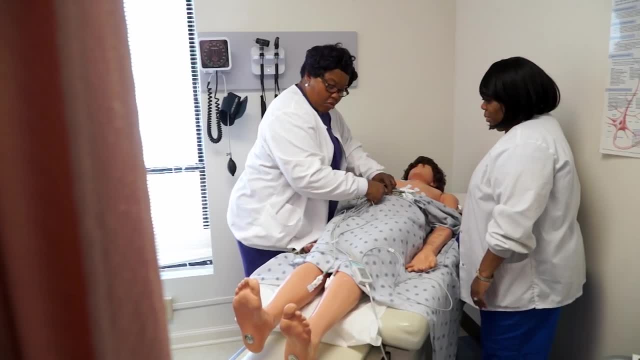 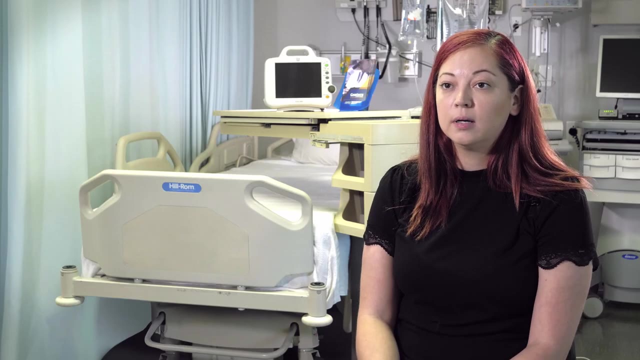 I joined the Army as a Biomed Tech about seven years ago and I enjoyed it and I wanted to continue it after I retired. Biomedical technology is basically the equipment and how we upkeep it and how we make it work. When it is hooked up to patients or your family or yourself, you want to make sure that equipment is going to work properly. 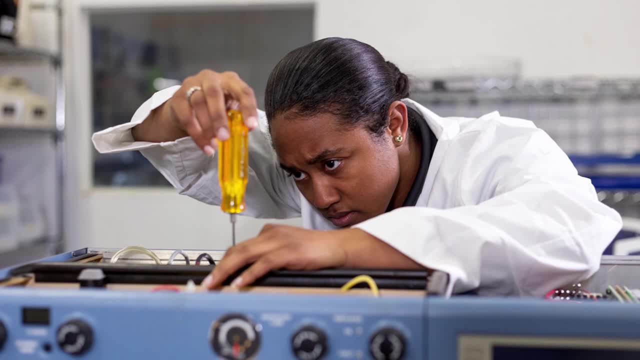 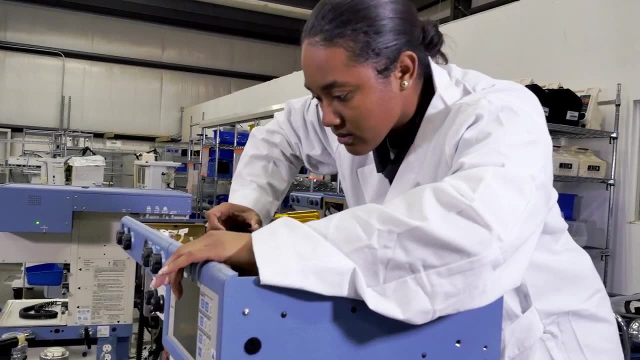 You want to make sure you do upkeep the equipment For preventative maintenance. we do also repair equipment. So a typical day for a Biomed student at Centura would be: either they're going to be working hands-on with the specific class's equipment. 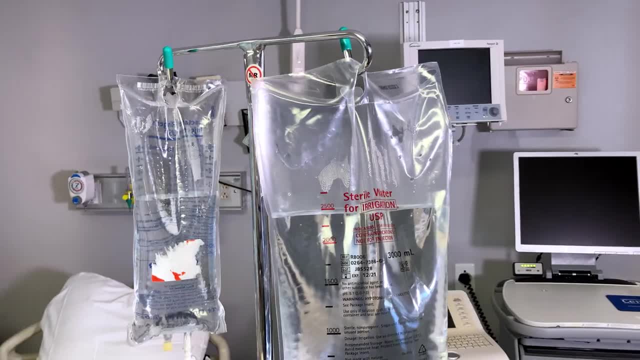 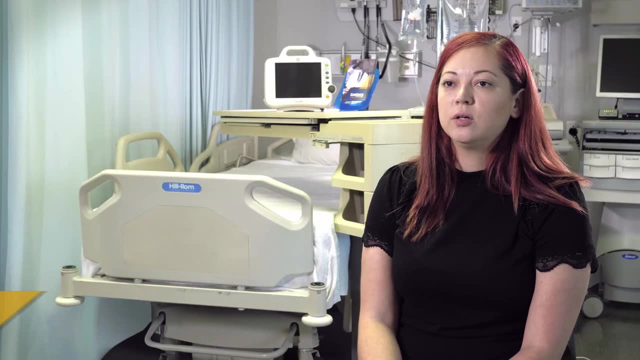 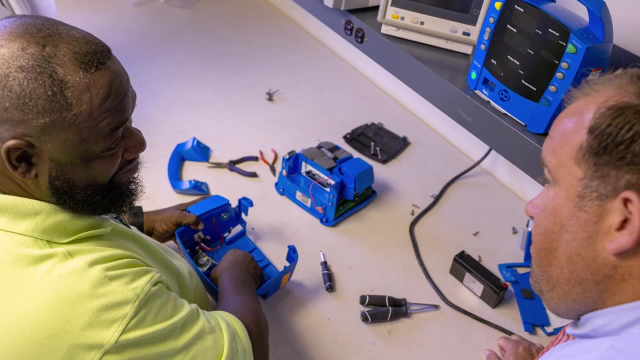 whether it's diagnostic devices or treatment devices. basic electronics, learning what the different components are, learning how to solder, learning how to troubleshoot. An ideal student for the Biomed program would be somebody that likes to solve problems, so somebody that can work in a fast-paced environment and is a good team player. 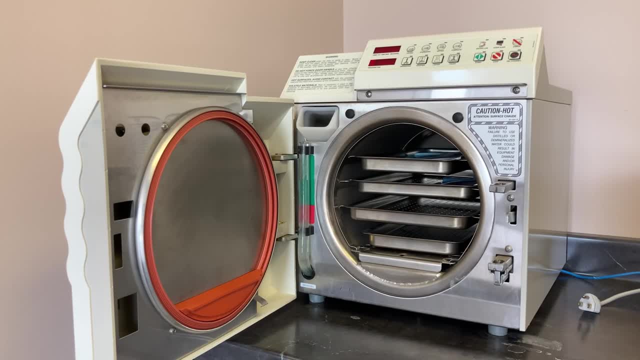 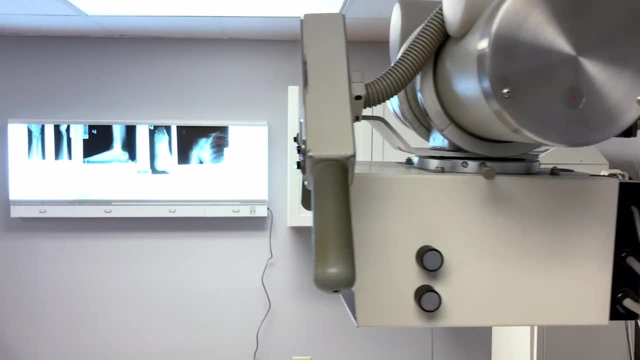 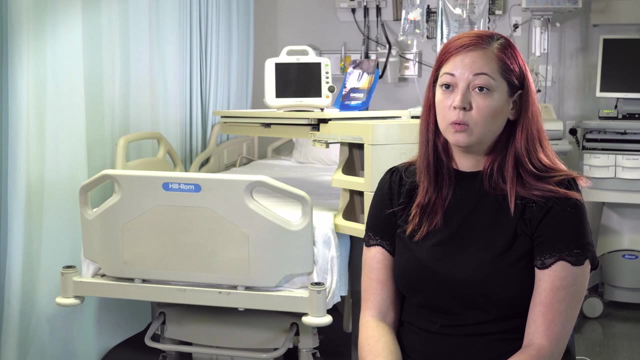 Biomed Techs also work on incubators and fusion pumps, respirators, ventilators, anesthesia machines. We work with all types of hydraulics. So somebody that goes through a Biomed program can expect to be a technician or a field service technician or work in a hospital. 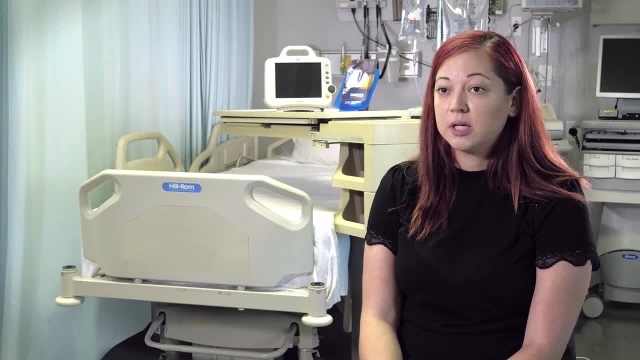 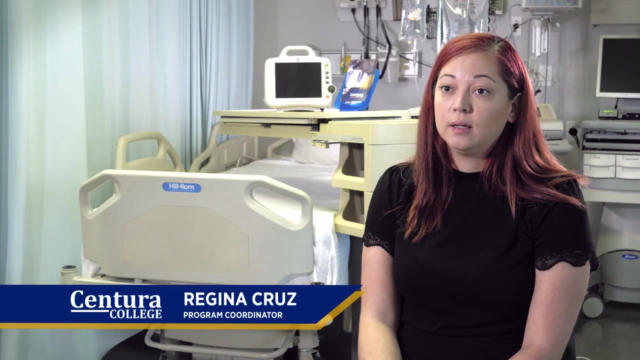 or work in small clinics or specialized clinics like dialysis or dental Or labs or even veterinary clinics. You can also be a health technology manager, meaning you would be over the Biomed Techs. Being a Biomed Tech is essential because without us, there would not be the ventilators or respirators that have been so important on treating these patients. 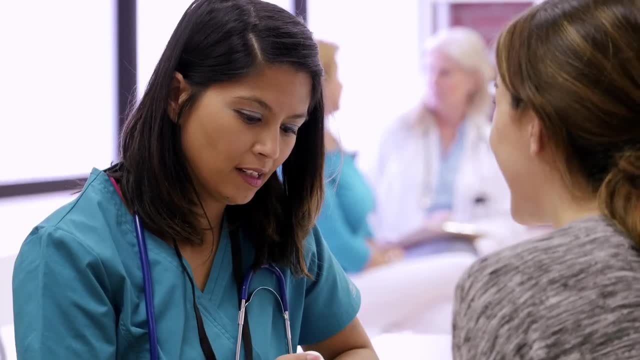 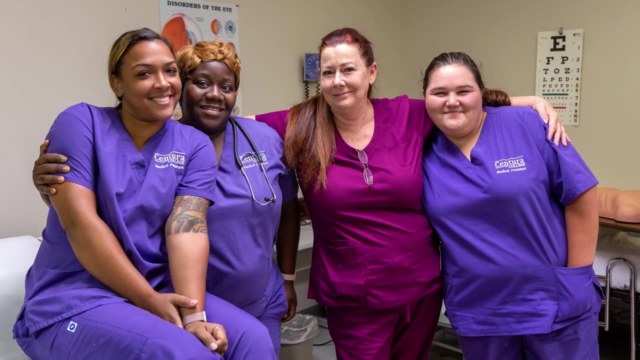 I have friends right now that have been working overtime just to make sure they have the ventilators that are needed in their hospitals. I love the Biomed field because I feel like we do make a big difference. Without us, there is no healthcare.